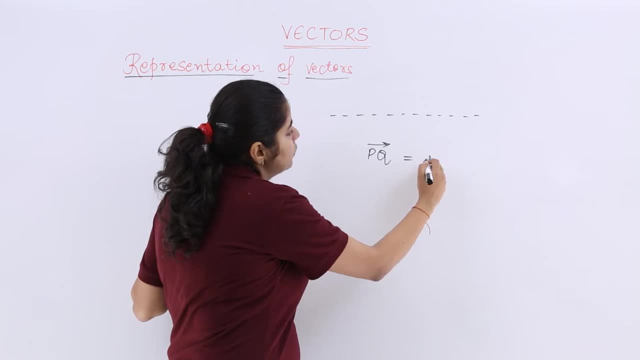 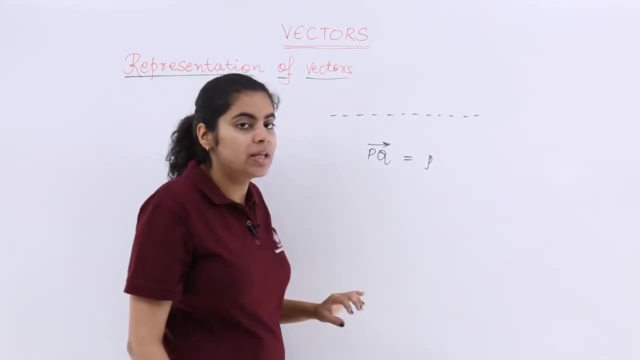 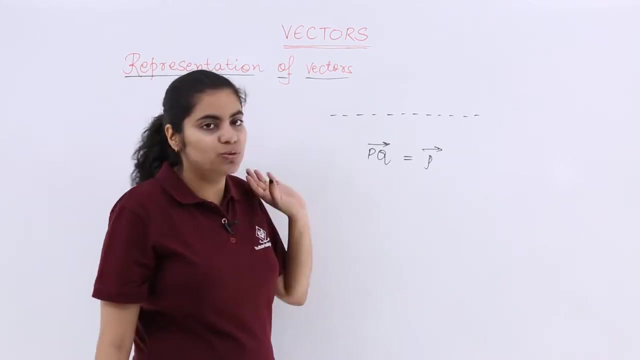 this PQ can also be named as: So if you want to name a vector using small alphabet, only one alphabet is sufficient Arrow should be made. but if you want to show it using two alphabets, then you have to use capital letters and those two should be there. The other thing, PQ, is equal to P vector. 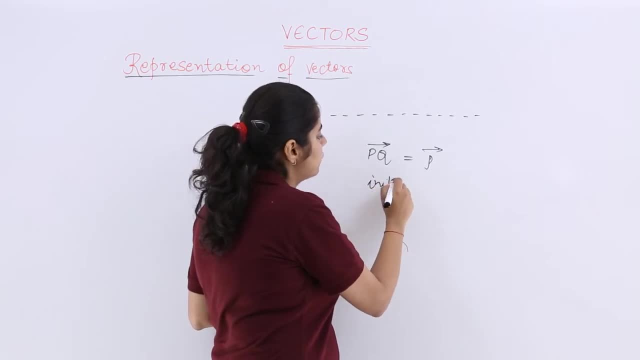 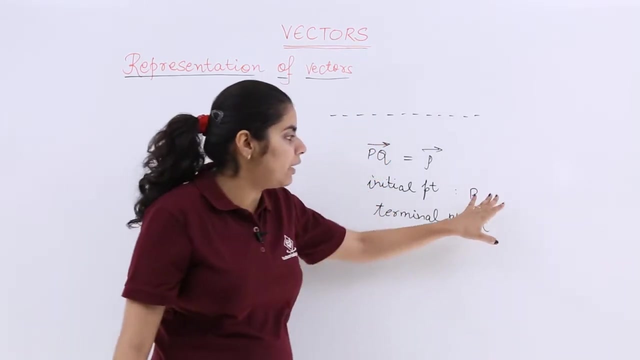 Now, PQ means the initial point as well as the final point, which is known as the terminal point. PQ is very much important to know. The initial point is P and the terminal point is Q means the vector, direction or sense is from P to Q. See three important terms that I will talk. 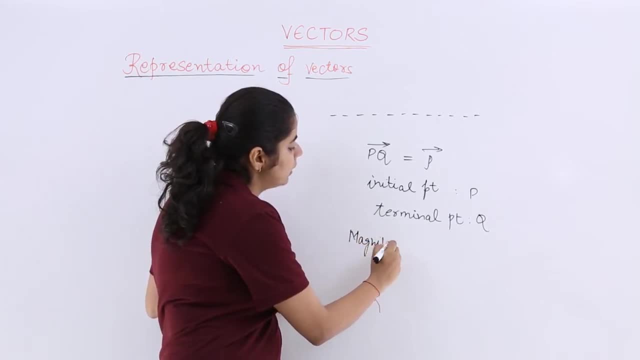 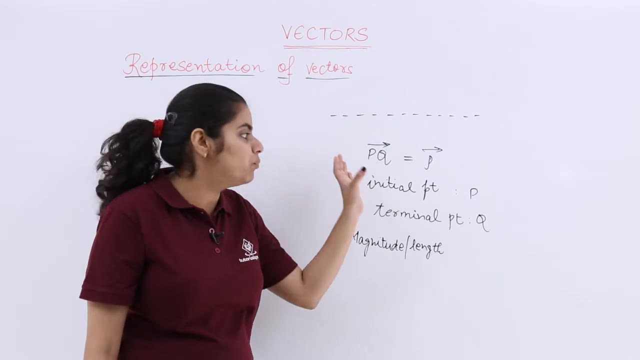 about One is your magnitude of the vector. Magnitude of the vector is also called as the length of the vector, and that is nothing but the distance from P to Q or between P and Q. So if this is an unlimited line, and I say this is an unlimited line and I say this is, 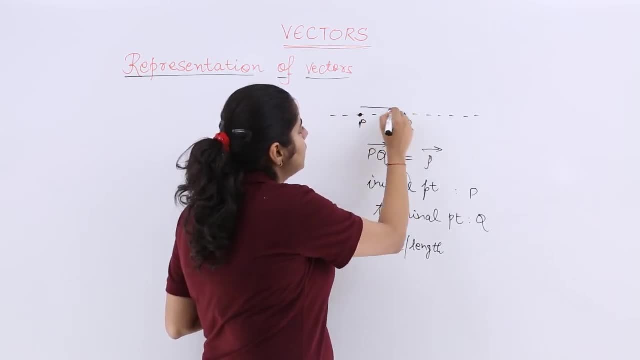 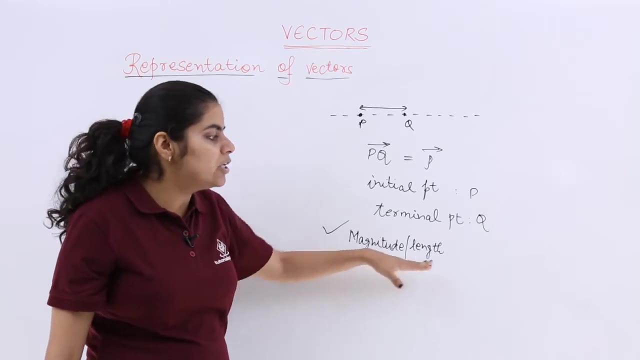 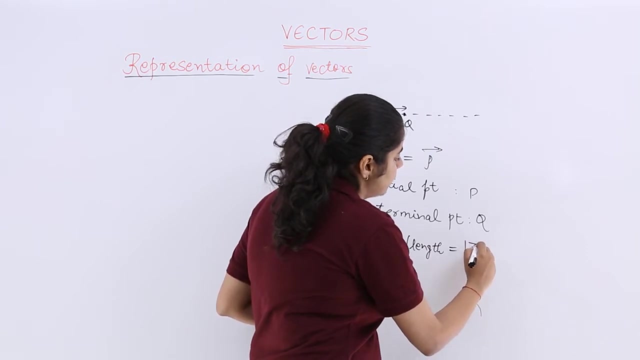 your point P and I say this is your point Q. then what is the length? whatever is the distance from P to Q? So that is the talking about magnitude or length. Now the magnitude or length is mentioned as if it is small p. So I will just say that magnitude is the modulus of P. that means it is never negative, or simply. 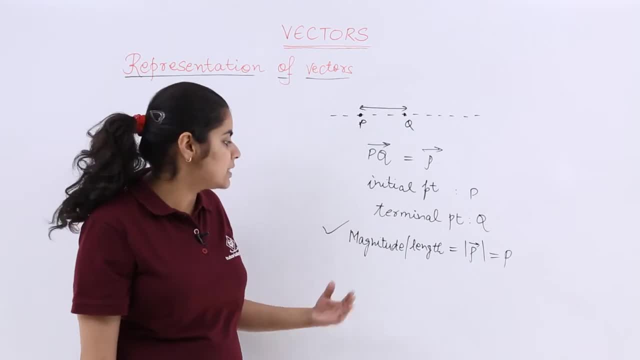 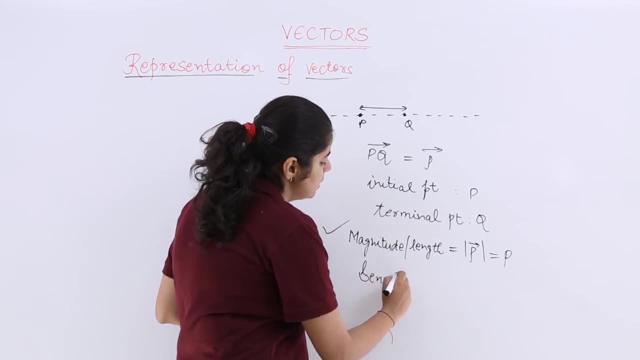 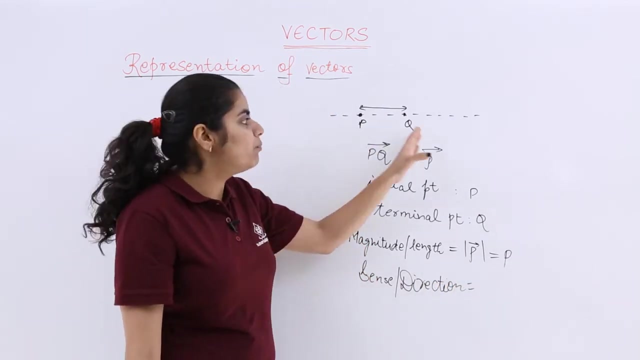 I can write. it is small p. Now, next is about magnitude and length. if I have done, I will talk about the sense. the sense is also called as the direction. now, what is the direction? when I go from P to Q, I say the direction is from P to Q. if it is the other way round, 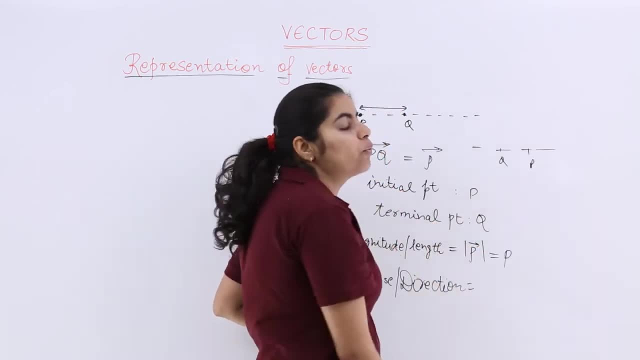 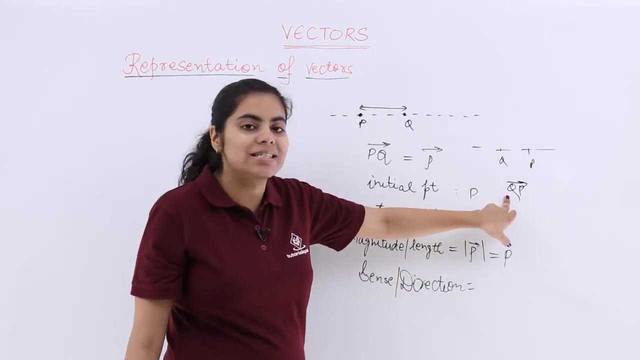 if you have a diagram like this: this is Q, this is P, and I am going from Q to P. I will write Q first, then P, so the first thing that you write is called as the initial and the next one is known as the terminal. last but not the least, but not very important also,